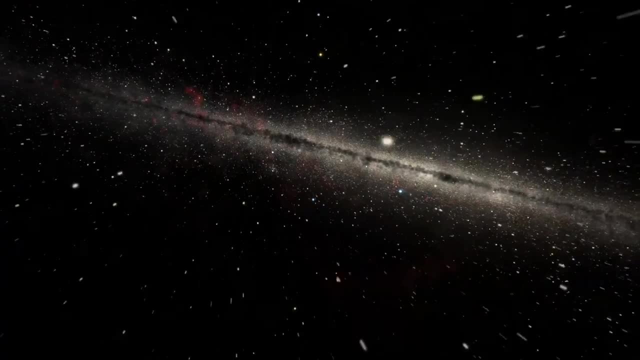 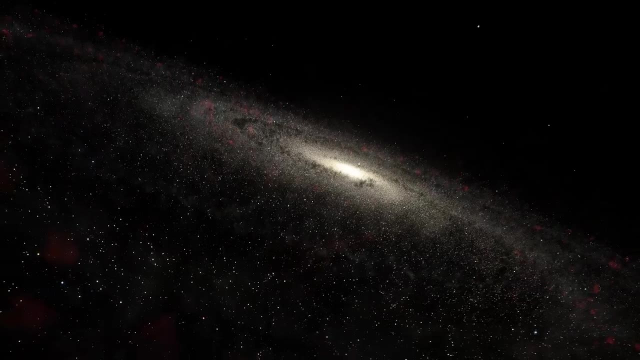 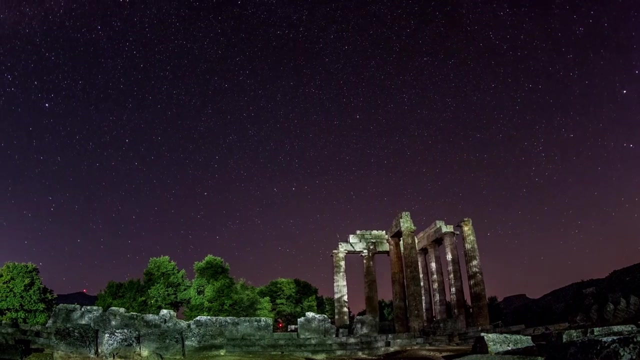 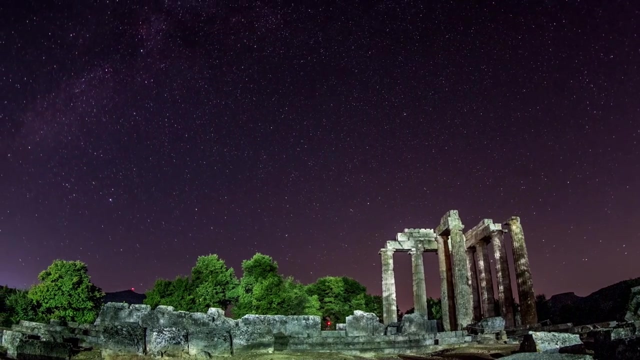 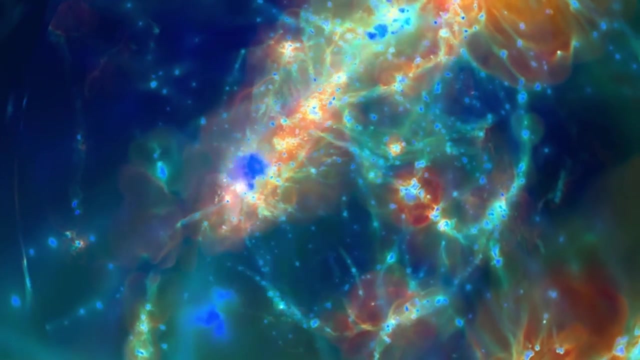 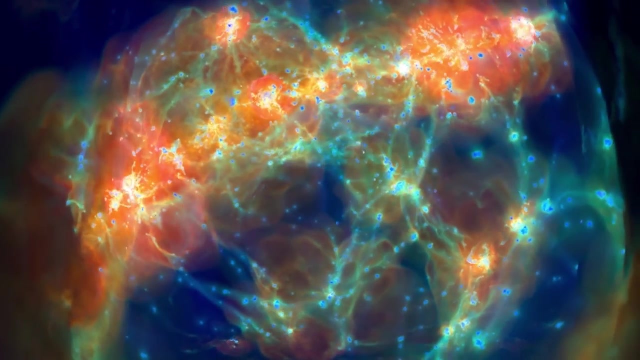 The universe was always the final frontier of the human quest for knowledge. Through all its history, humanity has observed the sky, trying to understand the cosmos outside the limits of our planet. Today, this effort has yielded significant results, especially in the study of high-energy astronomical phenomena. 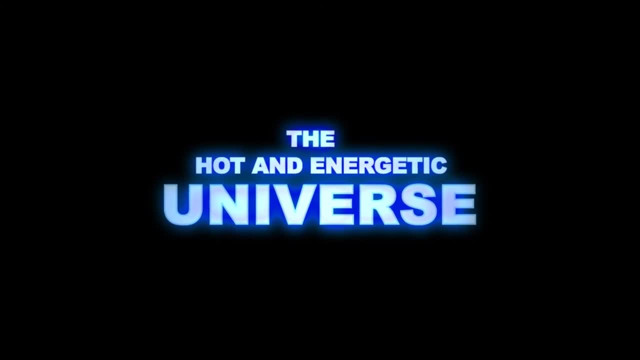 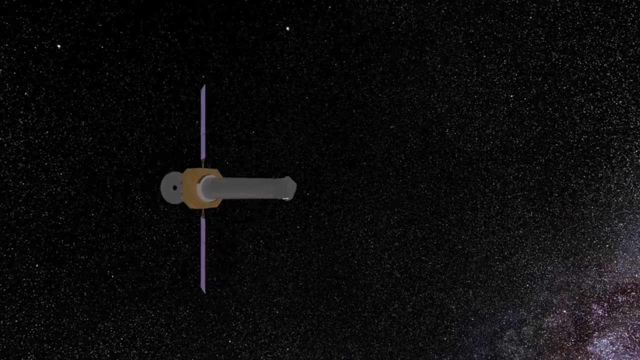 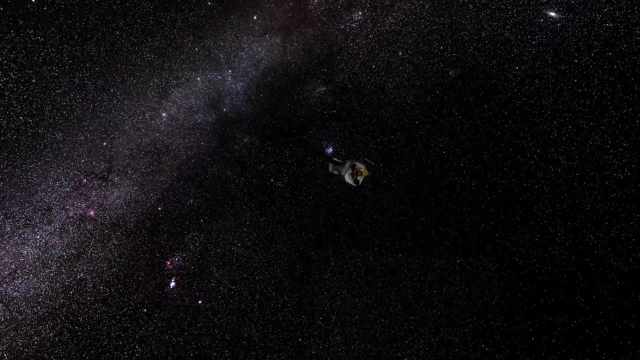 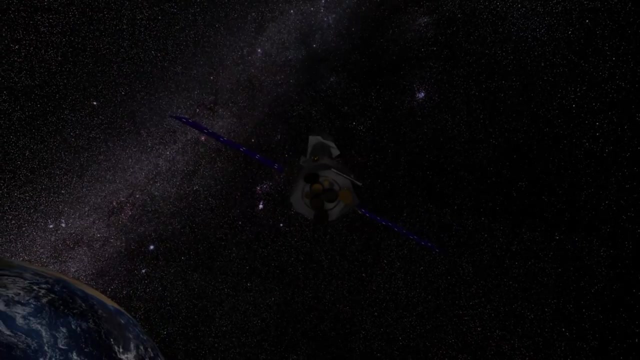 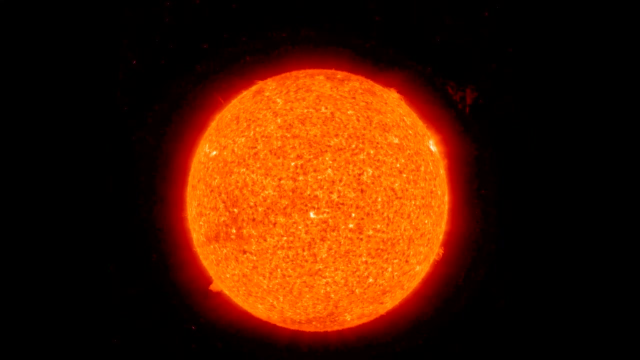 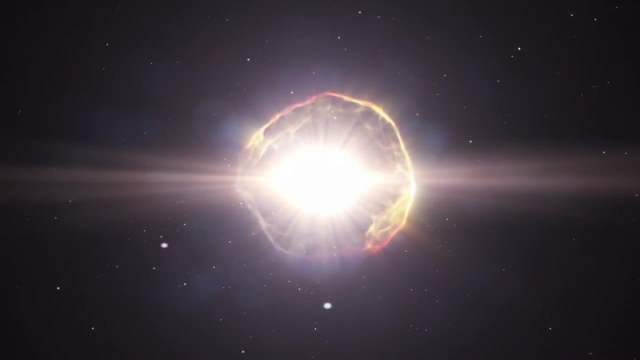 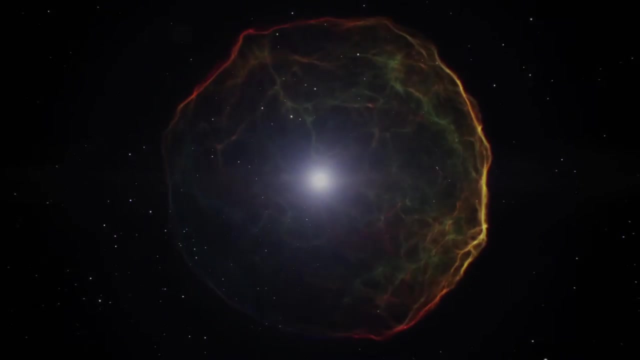 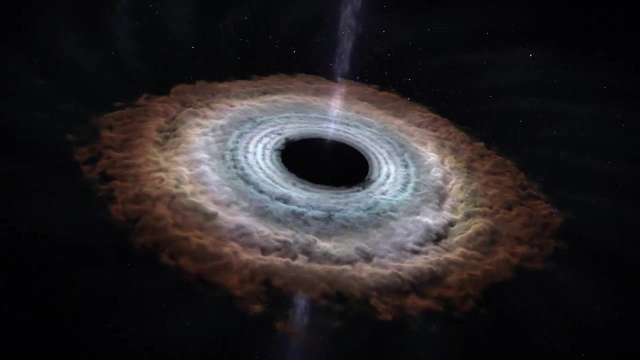 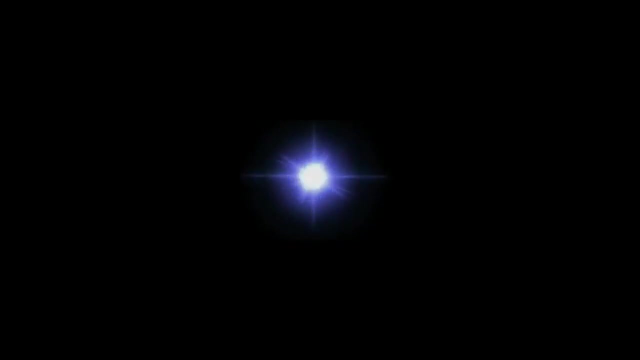 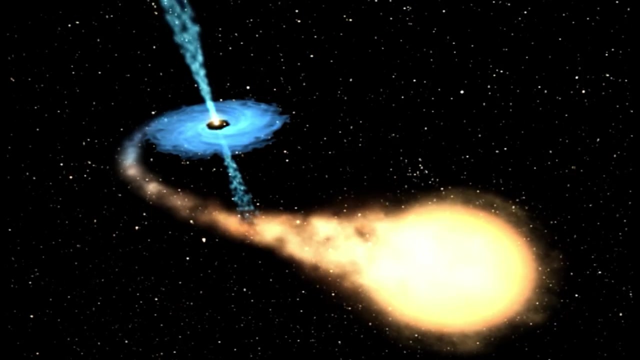 The only way to observe the hot and violent universe at high energies is to use observatories in space. With these observatories we study in detail The active sun, Supernova eruptions, Black holes and their environment Pulsars. We also observe binary stars that are very close together and interact strongly with each other. 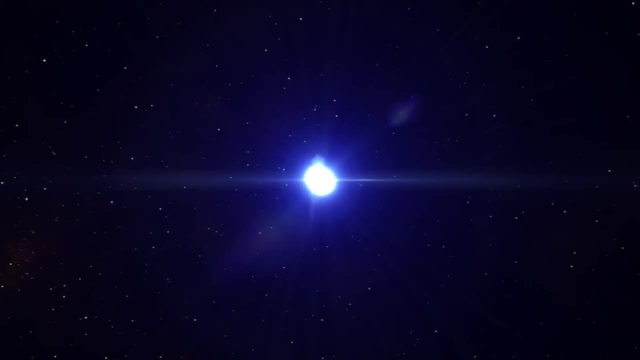 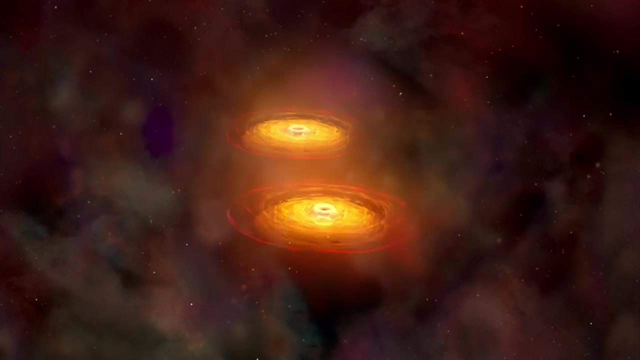 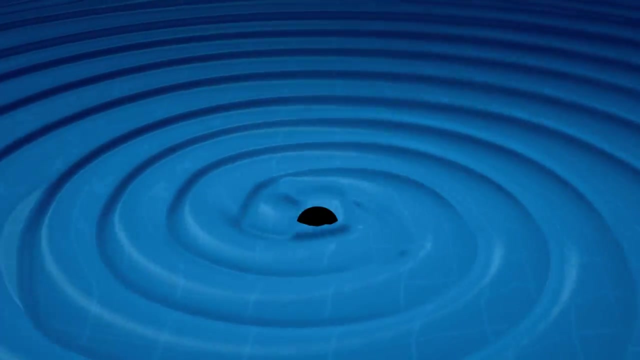 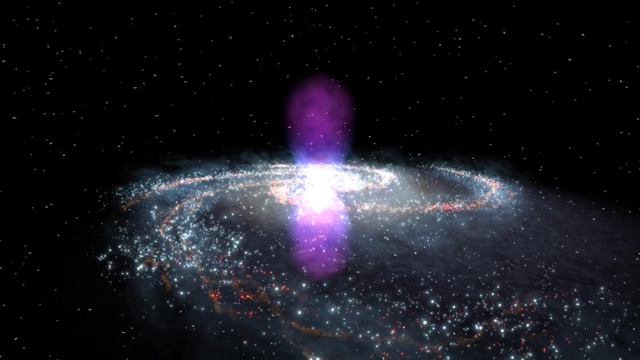 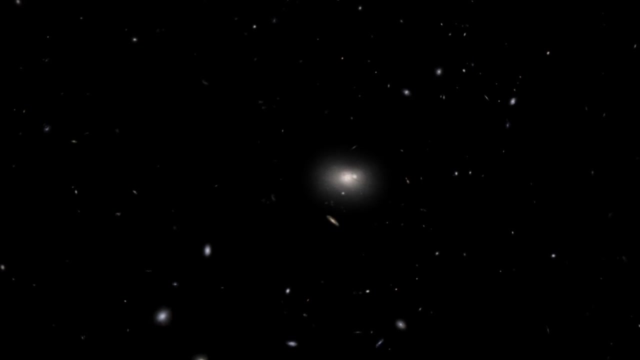 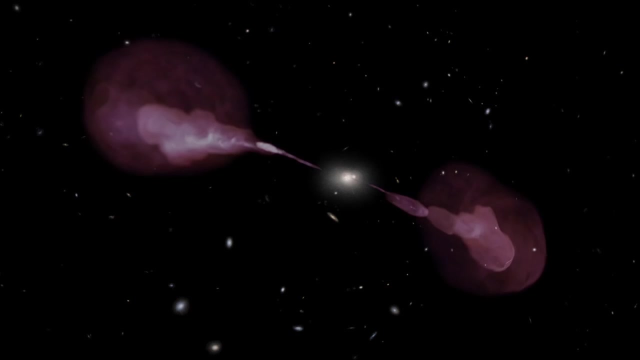 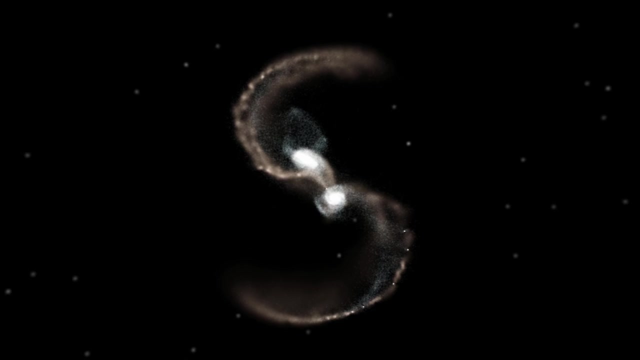 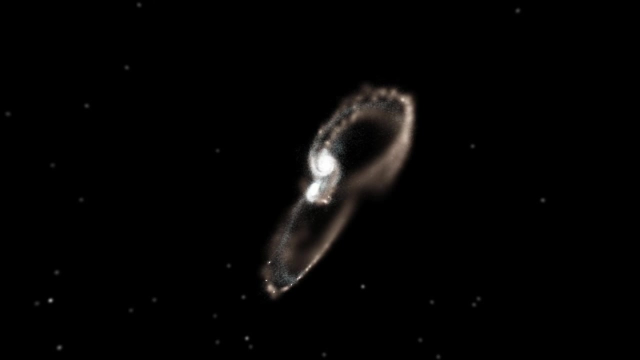 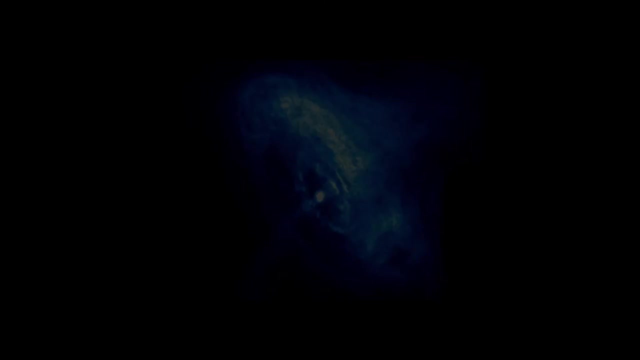 The merging of neutron stars, The merging of dwarf stars, black holes, the violent center of the Milky Way radio galaxies, quasars and blazars galaxy mergers, the universe seen in X-rays and gamma rays in an inhospitable and violent environment.